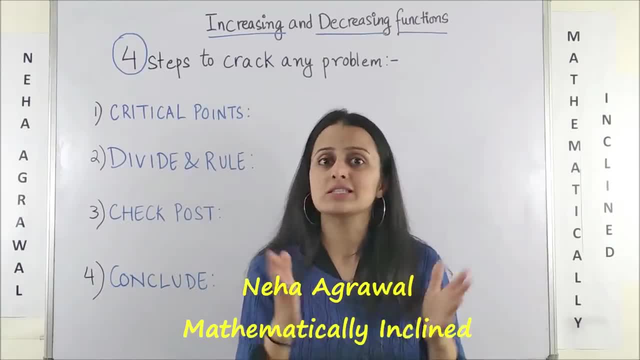 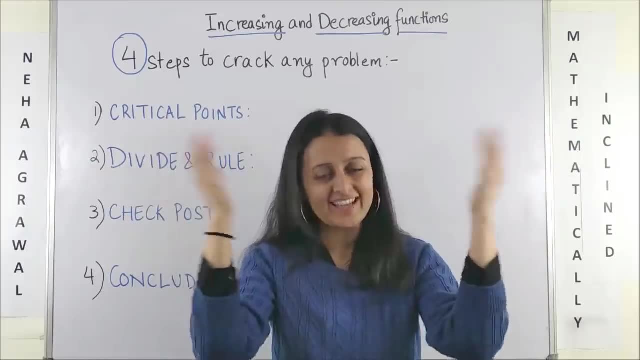 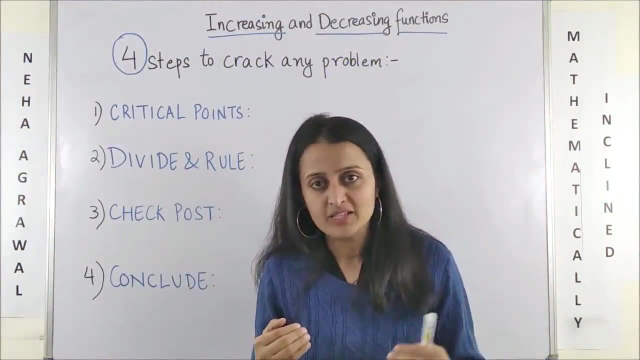 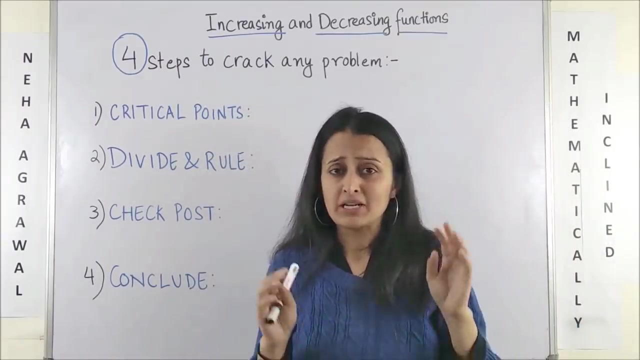 Increasing and decreasing functions for CBSC, ISC and state boards. Four steps, four marks in. Are you excited? Let's get started. So we usually expect a four marker from this portion, and what I have done is I have divided everything into four simple steps. Just remember these four steps, boss. You can crack any question. 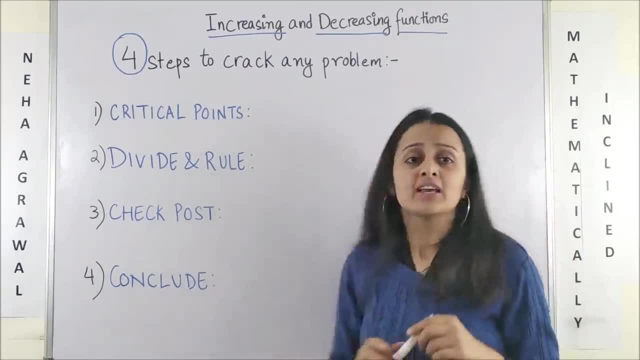 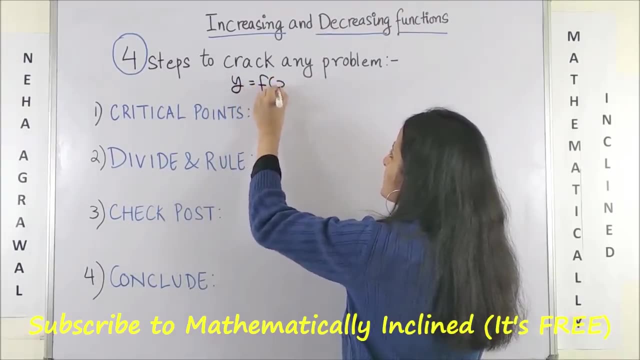 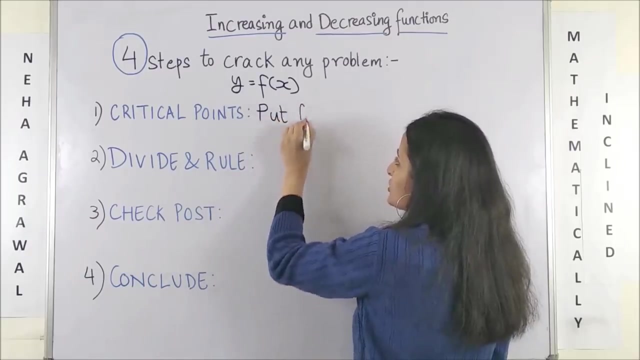 in increasing and decreasing. So step number one, critical points. We all know this. If you are given a function, y is equal to fx. then step one simply says: critical points means: find your f dash x, that means the derivative of the function, and put it equal to zero. 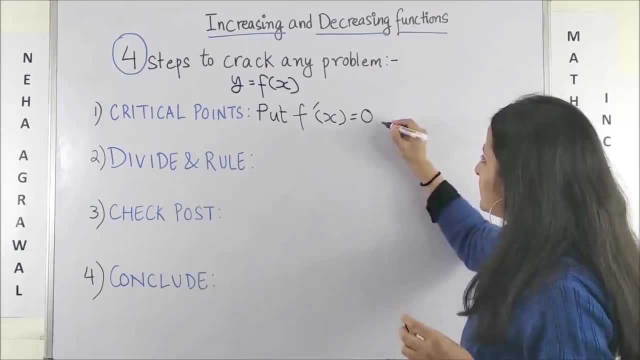 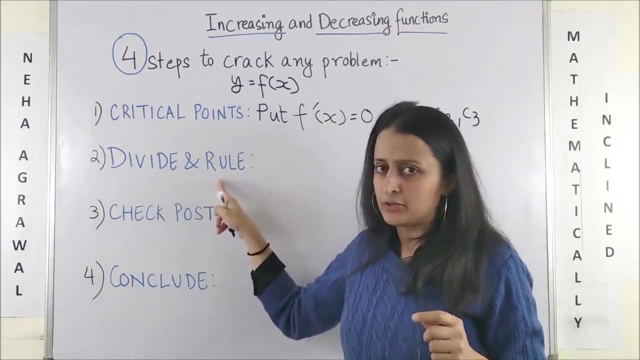 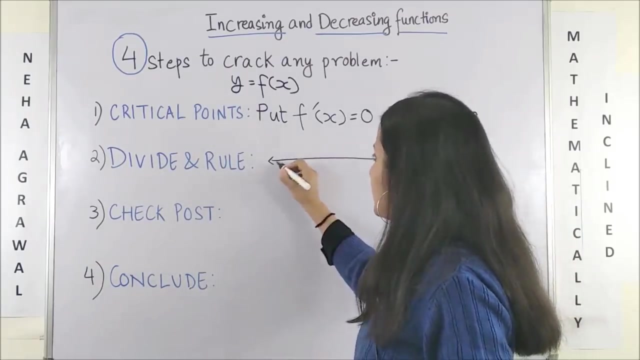 Hena. simple, Suppose we end up getting the critical points to be, let's say, some c1,, c2, c3.. Next step is divide and rule Always works. What you do is now suppose you are given an interval. Let's say a to b. Please note: if no interval is given to you, then the interval 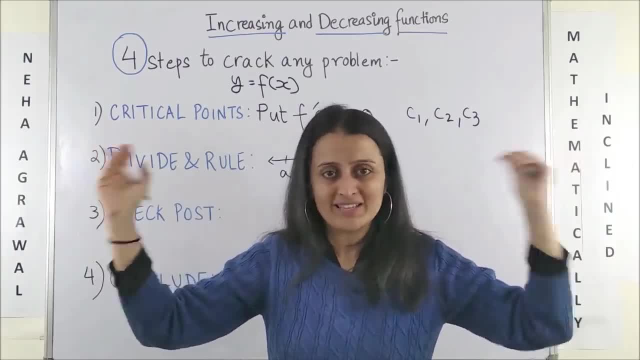 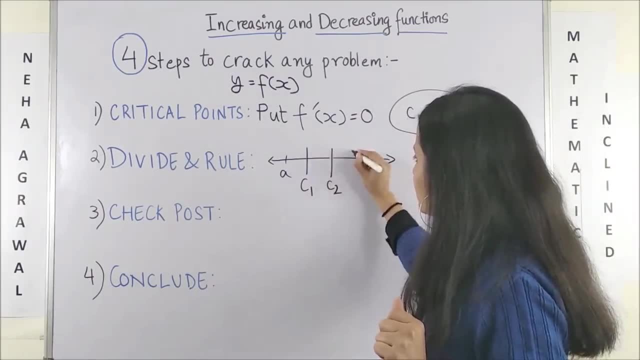 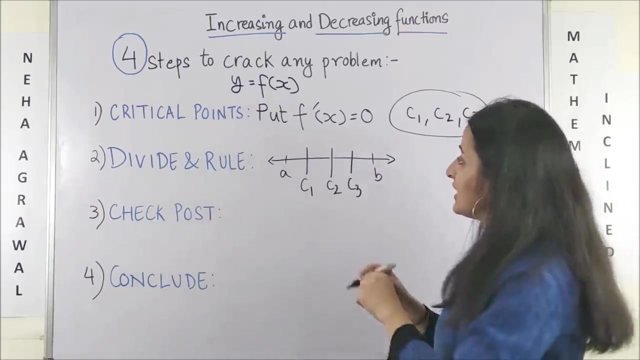 is the entire real line, minus infinity to plus infinity. Now what you do is, in ascending order, split or divide your interval, given interval into shorter subinterval. So divide and rule. Now you have created 1,, 2,, 3, 4 subintervals in the process. Step: 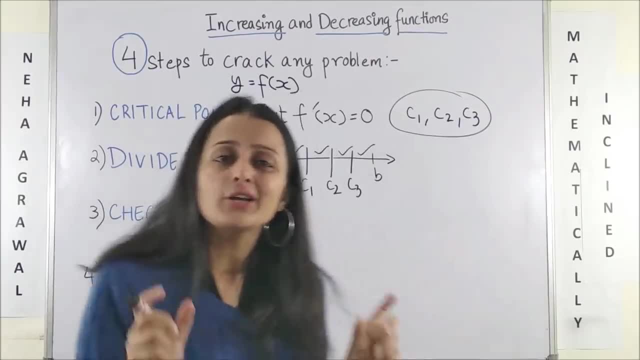 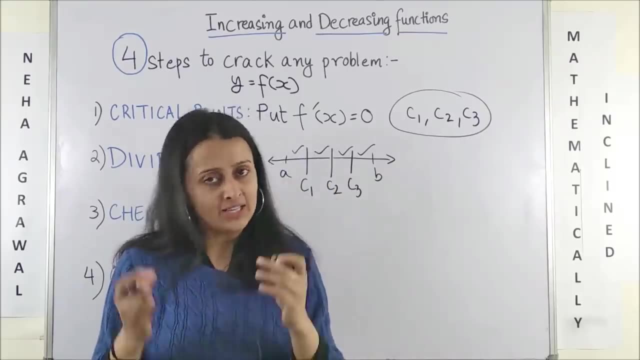 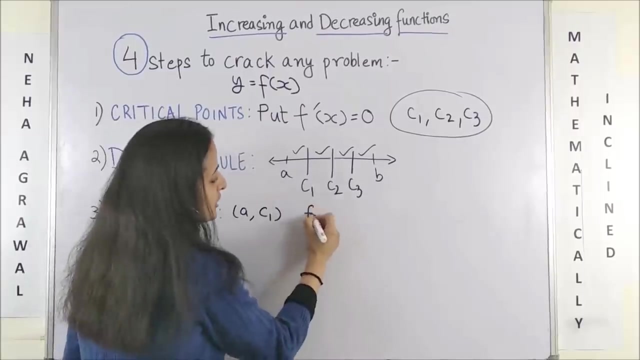 number three, the check post. Yes, here you check for the signs of the function or signs of the derivative for every subinterval. Toh kya karna hai, boss. Like the first subinterval is a to c1,, you would check for the value of. 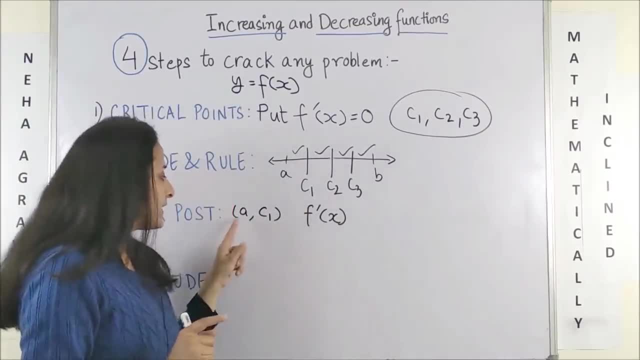 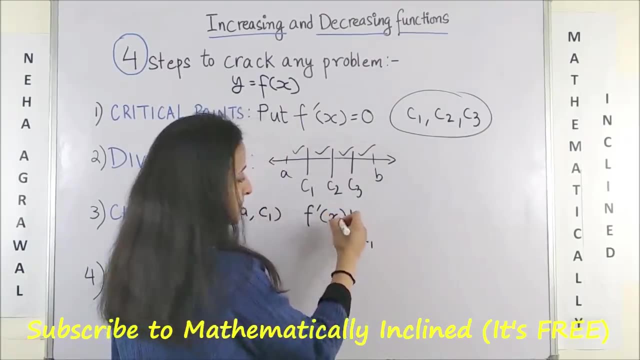 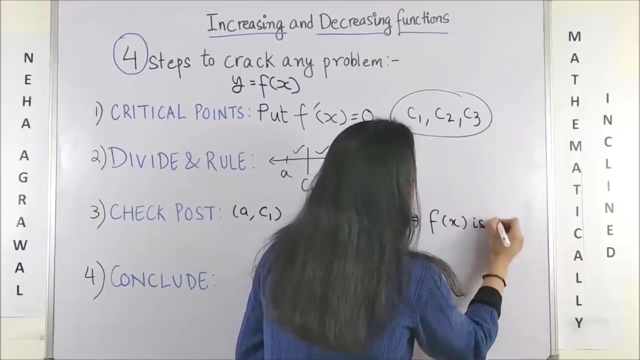 But where will you check? Simple: Take any point lying in between this interval. So take any point. let's say you choose something like an x1, substitute. If it turns out to be greater than 0, this means the function is increasing in the interval a to c1. 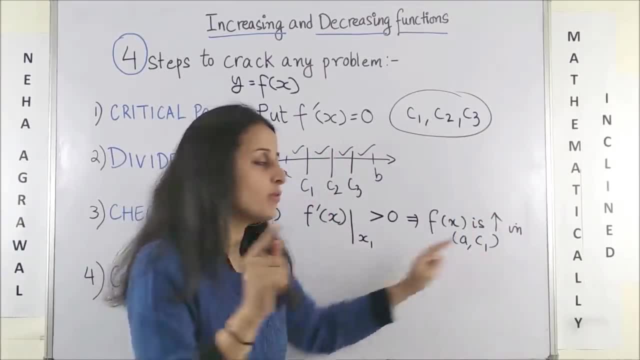 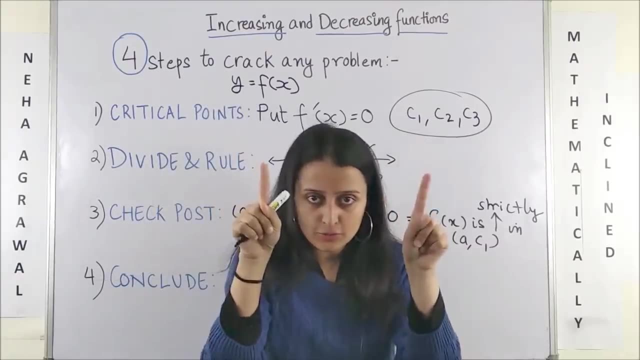 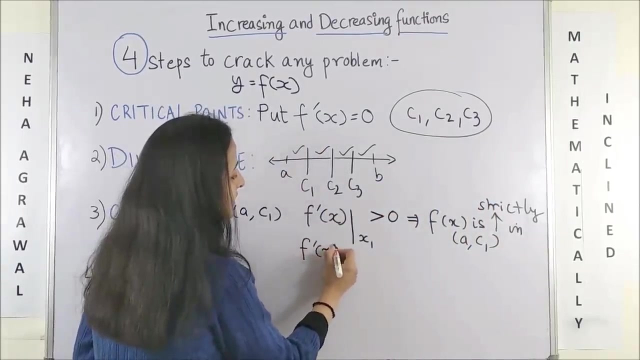 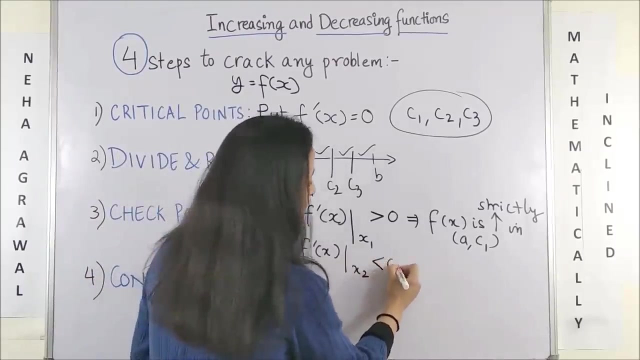 Please note, since the intervals you choose to be open to is increasing- ko keh dena, strictly increasing. And in case you choose the intervals to be closed brackets, then you will say simply increasing. Same way, if let's say for the next interval it turns out to be, let's say some point I take in between which gives us less than 0, then obviously this means fx is strictly increasing. 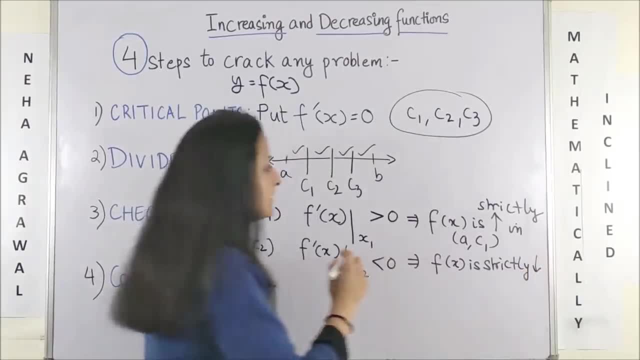 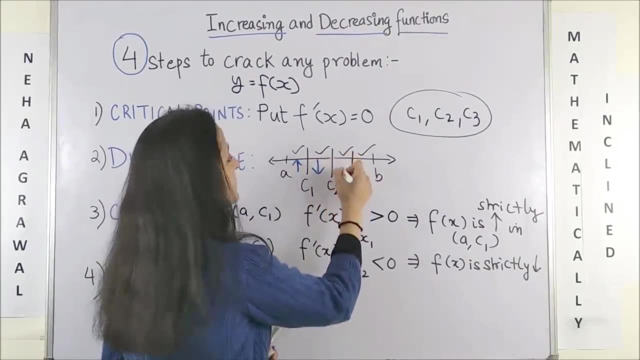 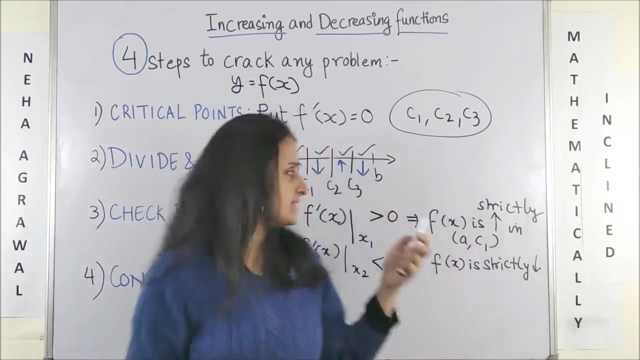 Decreasing in the given interval. Saath saath, for your convenience, keep putting the signs. Let's say this is increasing decreasing. maybe the next one is increasing decreasing. Now, most of us know that in 99% of the cases, the signs always alternate. 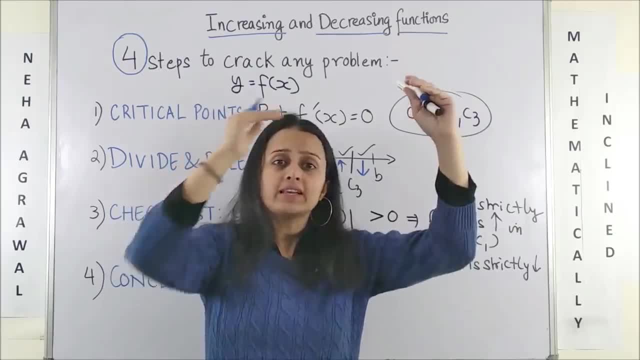 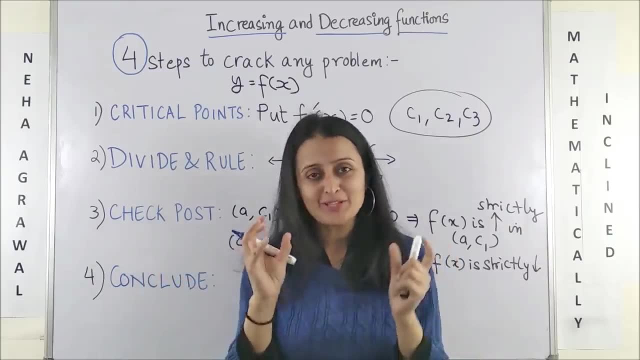 Agar increasing hai to next decreasing hai, fir increasing hai next decreasing hai. However, don't assume What if you get points of inflection. Points of inflection are simply where you end up getting the same sign: Jaisa yahan increasing to yahan increasing. 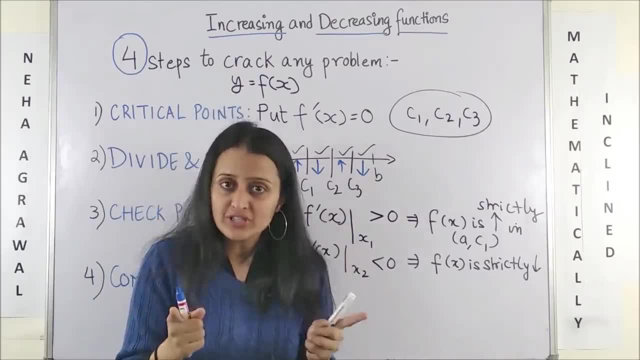 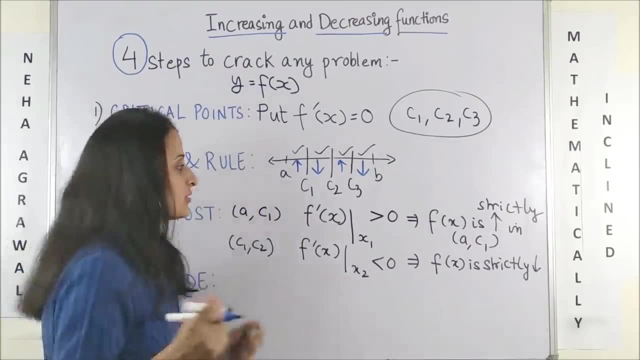 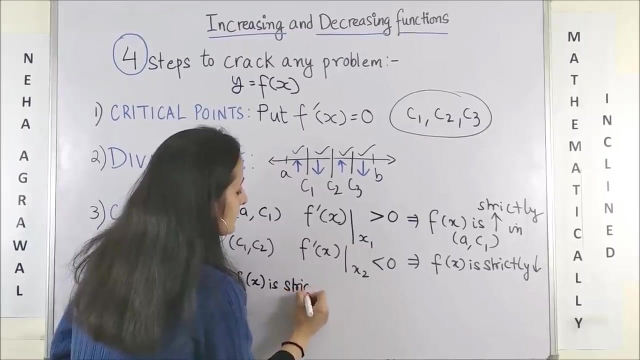 To c1 banjata hai point of inflection. So do check for each sub-interval. Itni jaldi mat karna. Now, coming to the last step, obviously conclude. So suppose this is what we got. So we will conclude by saying function is strictly increasing in the interval. let's say: 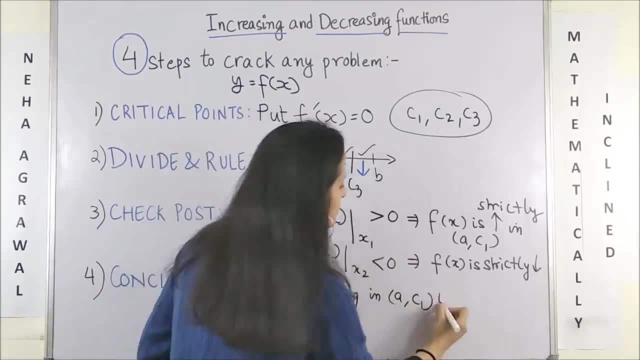 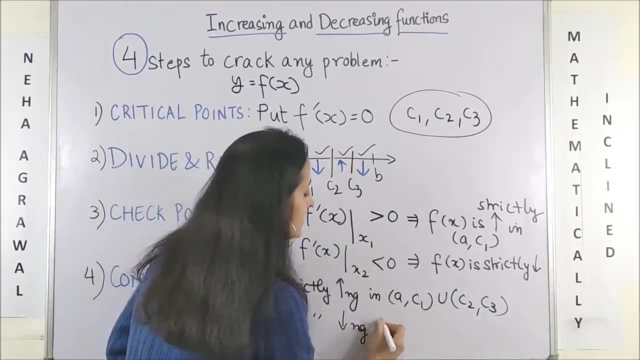 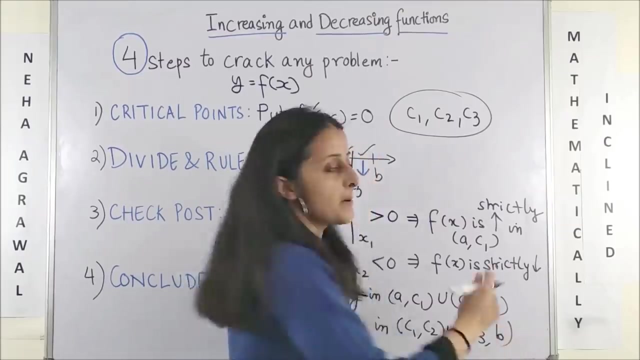 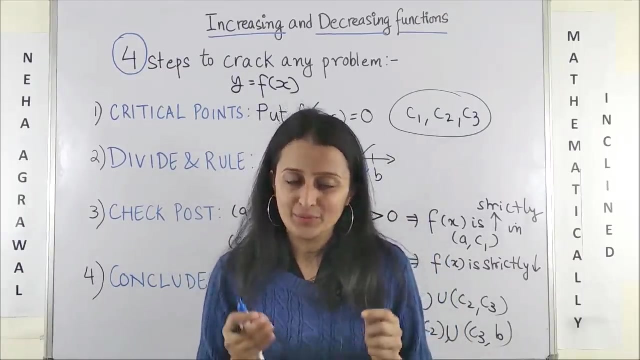 You have a to c1 and c2 to c3.. So this is how I write. and same way, function is strictly decreasing in the interval c1 to c2. union c3 to b. Bas itni si baat hai. Make a note, it is very important, and then I will move ahead with the questions. 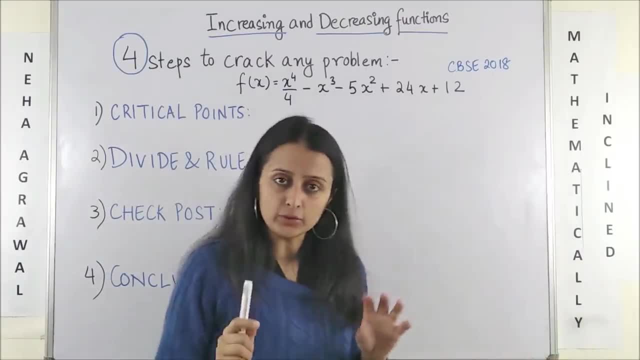 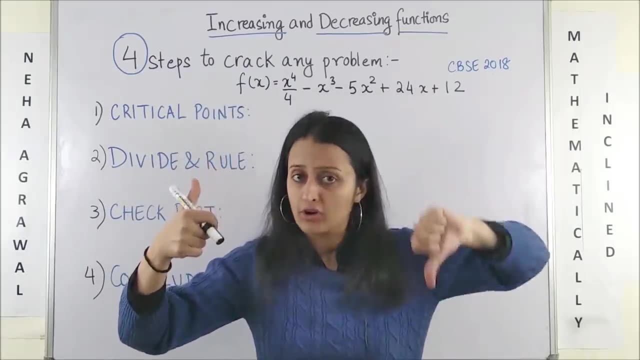 Please have a look at the question Question which came in CBSE 2018.. Question said: obtain the intervals where the given function is strictly increasing or strictly decreasing? There is no interval given to obvious hai boss. It will be the entire real line. 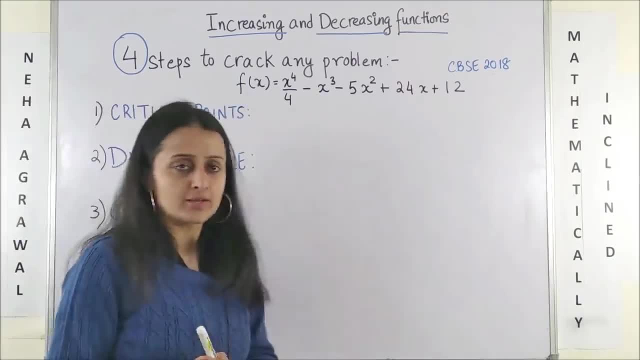 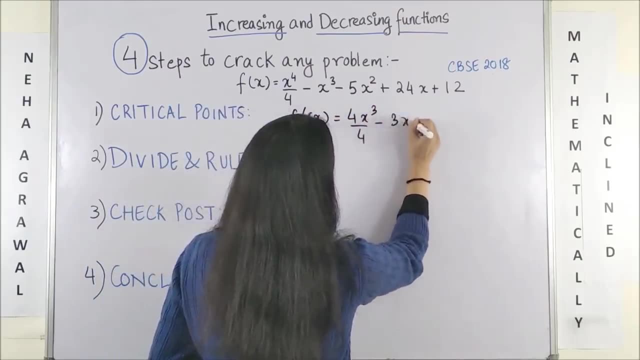 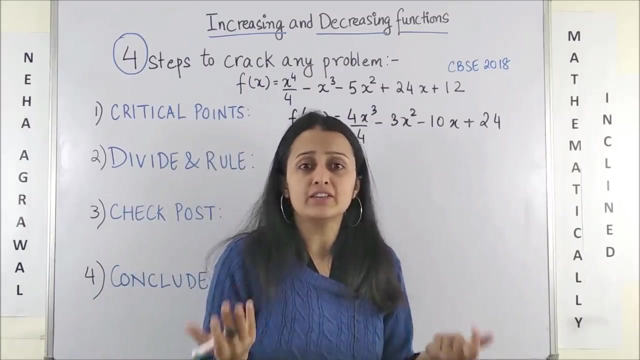 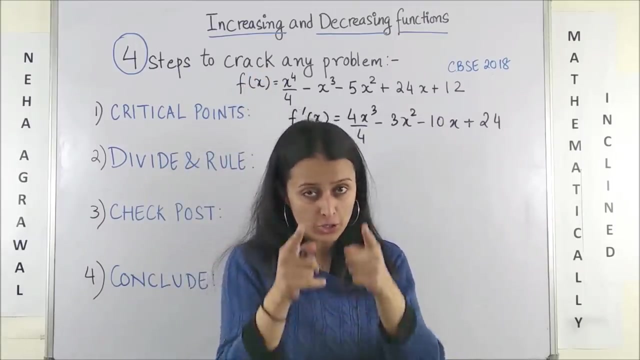 Now what we have to do is first step critical points. So I take the derivative which is 4x cube by 4 minus 3x square minus 10x plus 24.. Okay Now, if you have any confusion in derivatives or differentiation, click at eye button. I have the whole playlist on differentiation. 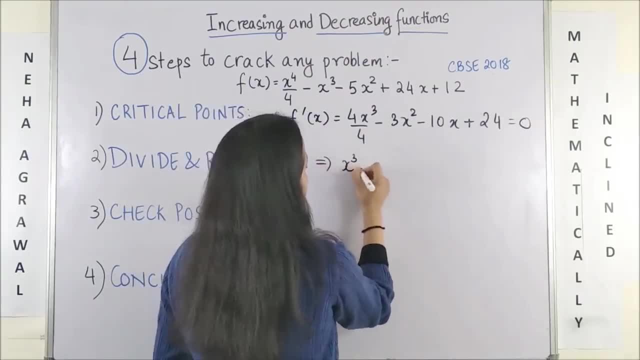 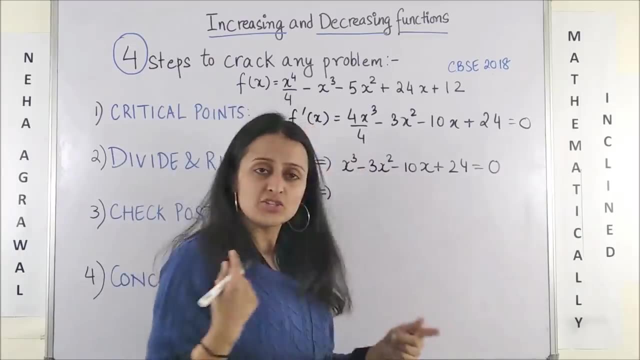 Do check that out. So that means now putting this equals to 0 gives me x. cube minus 3x. square minus 10x plus 24 is equal to 0.. Here now let's just get the factors for this. 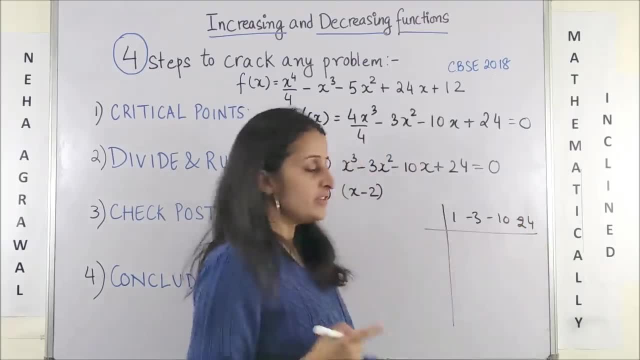 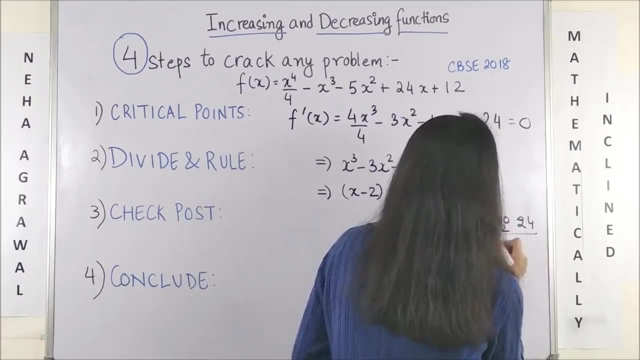 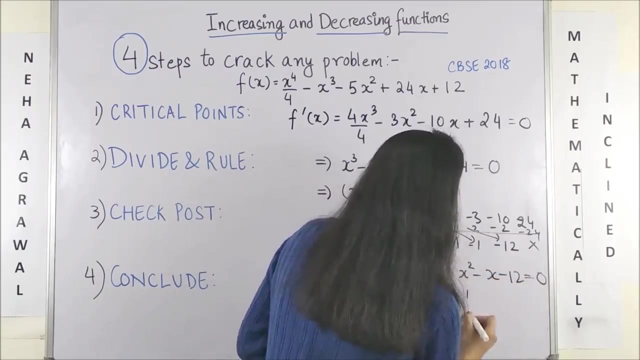 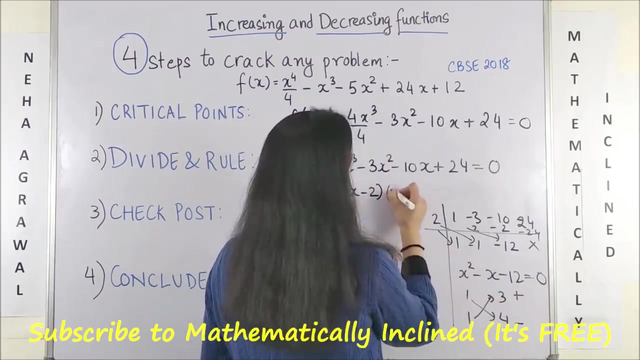 So, So, So, So, Now, Now. Now, One of the factors is x minus 2, and for the remaining I will have, I will get another quadratic which is x square minus x minus 12.. So the factors would be x minus 2, x plus 3 and x minus 4.. Now, if you are wondering, 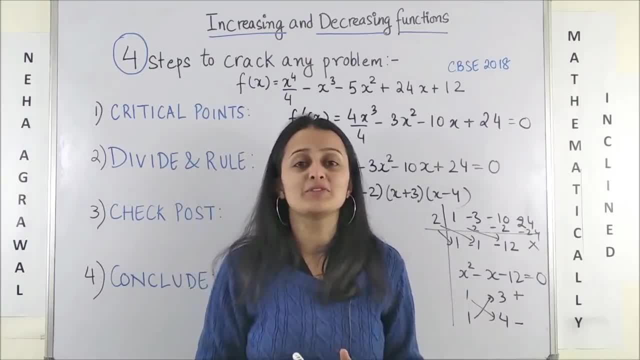 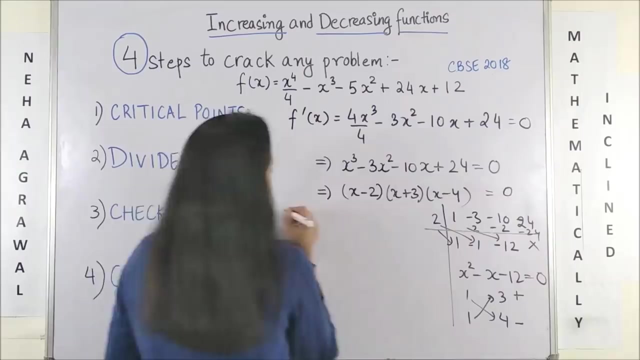 kiye kaisa jadu hua that you got these factors super fast. then click on the i button. look for my video which says cubic factorization in just 10 seconds. You will find the link in the description box also. So once we've got these factors, put them in, putting them equal to 0. 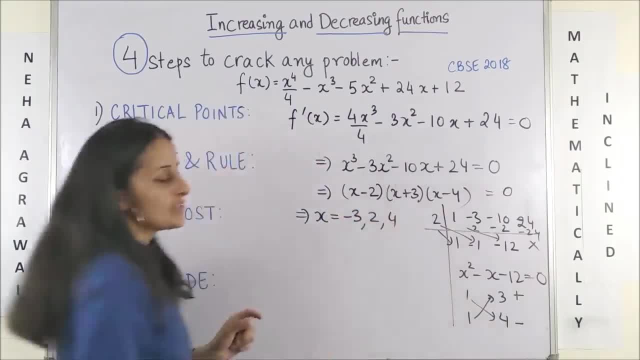 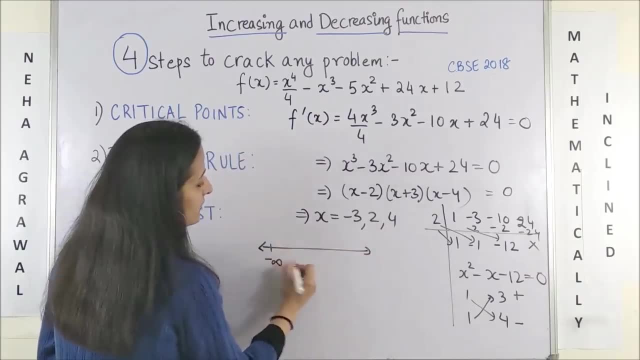 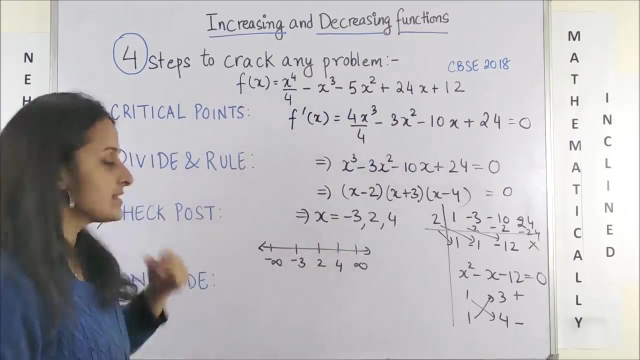 gives us x is minus 3, 2 and 4.. So now let's move to step number 2, which is divide and rule. So it says: since no interval is mentioned, my interval is minus infinity to infinity. I plot these in the ascending order. Now we have created some. 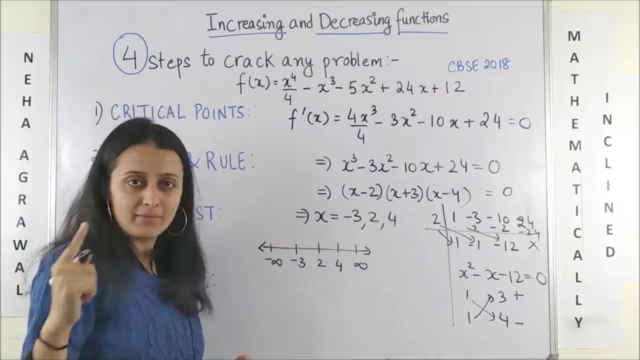 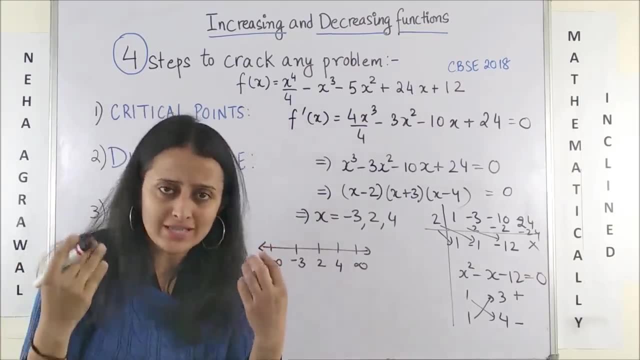 subintervals check post. So I'm going to check one by one on each of them. So f dash x on interval minus infinity to minus 3, choose any number, let's say minus 4.. So minus 4 pe. just put it here. 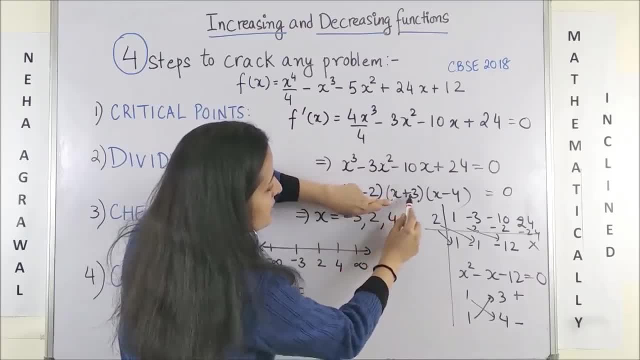 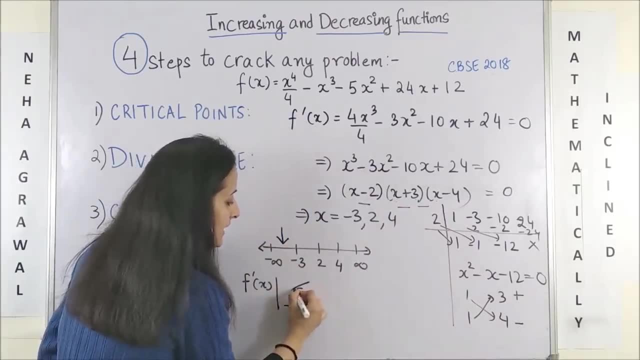 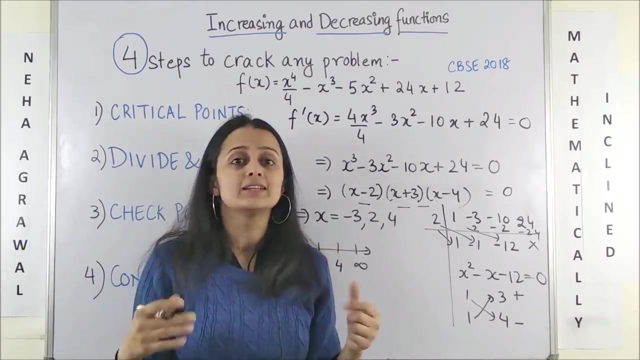 minus 4 minus 2 is negative. minus 4 plus 3 is negative. minus 4 minus 4 is negative. 3 is makes it less than 0 or decreasing. So we are not actually interested in the exact value, we are only interested in the sign, whether it goes up or it goes down. Same way looking at the next one, 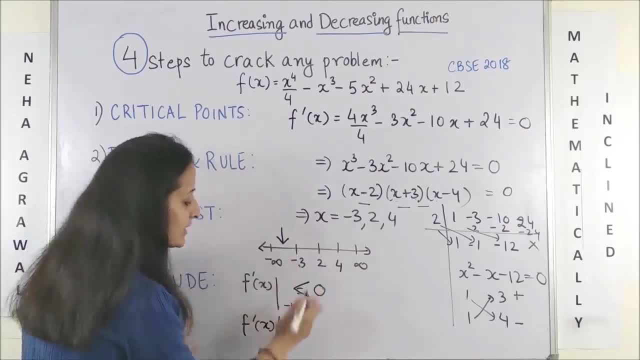 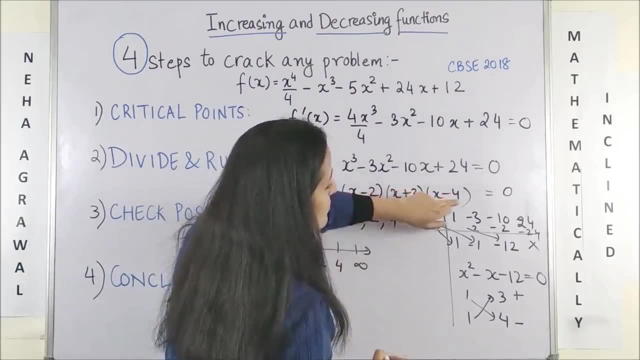 f dash x. at any point between minus 3 and 2 best is to take a 0. So 0 minus 2 gives me negative, 0 plus 3 gives me positive, 0 minus 4 gives me negative. So everything makes it positive. 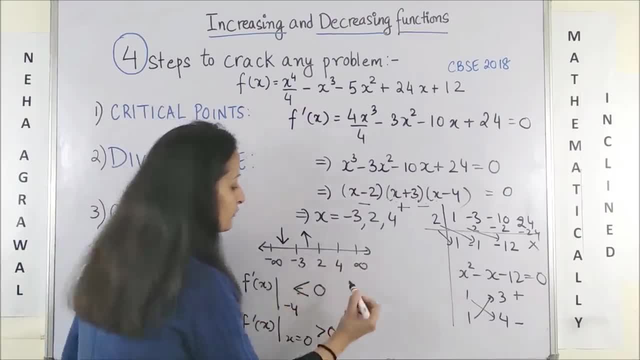 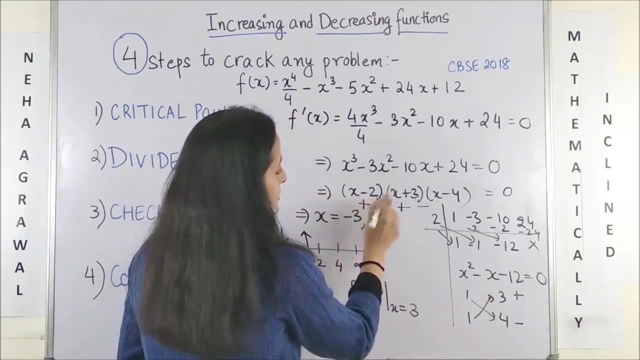 and the function is increasing Same way: 2 to 4.. So f dash x. simply, I can take 3.. So 3 minus 2 gives me positive, 3 plus 3 gives me positive, 3 minus 4 gives me negative. This is negative, and 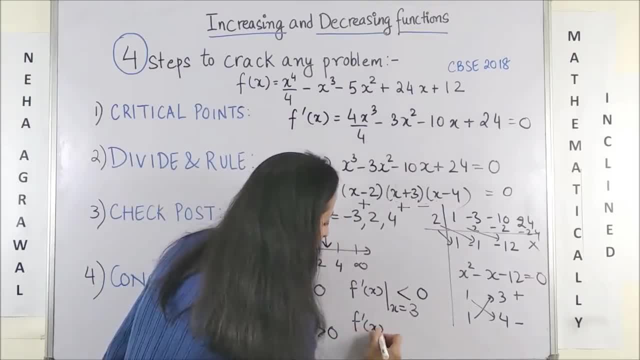 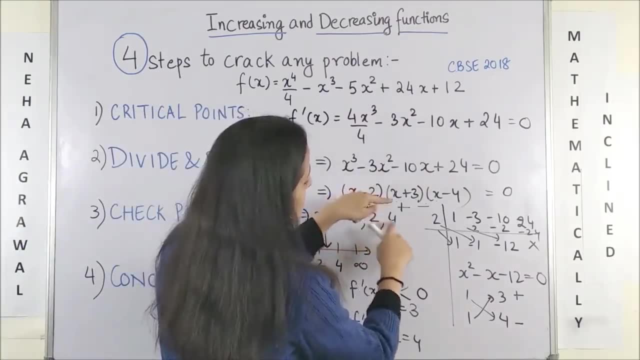 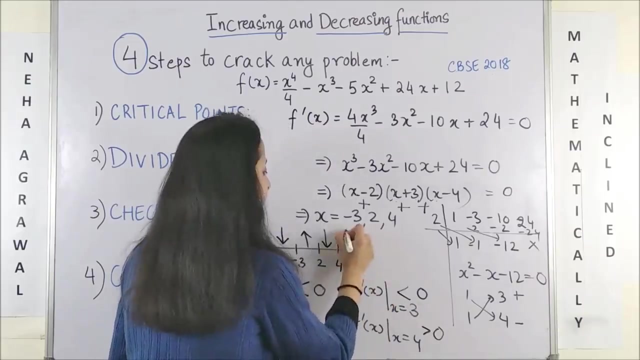 it is decreasing. Now, moving on to f, dash x at x equal to 4.. So I can choose, maybe 5.. So choosing 5. 5 minus 2 gives me positive, 5 plus 3 gives me positive, 5 minus 4 gives me positive. So overall it's positive and it's increasing. Okay, make a note. 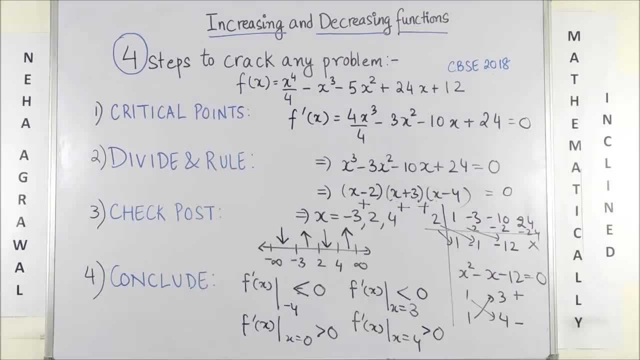 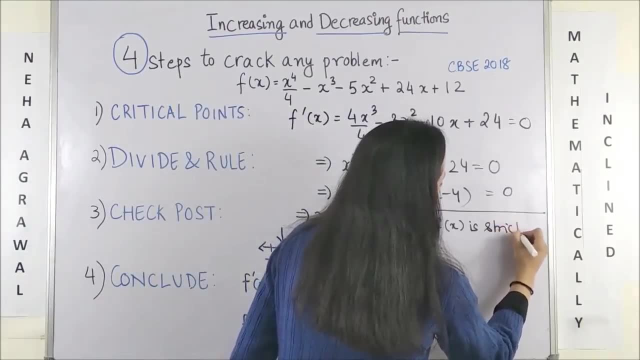 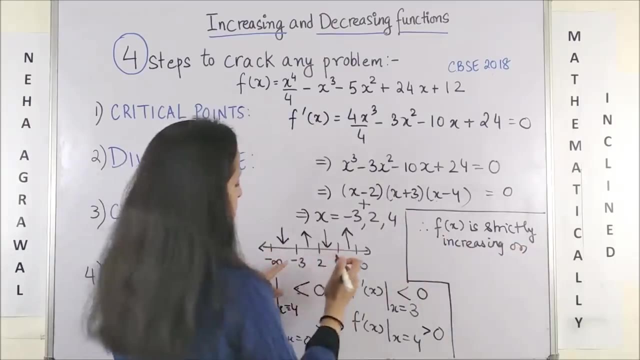 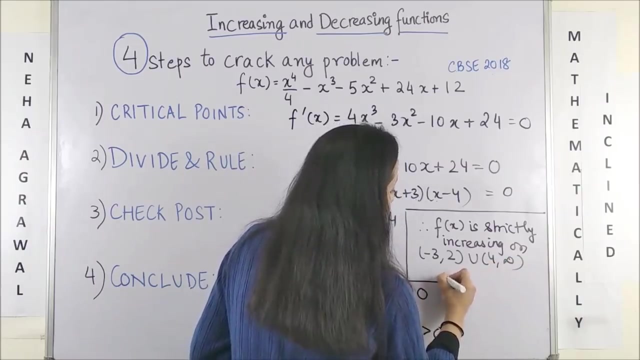 and then we will just conclude. So now I simply conclude: I say fx is strictly increasing. I mean you can write it completely On the intervals I can see minus 3 to union 4 to infinity, and of course fx is strictly decreasing on the interval minus infinity to minus 3, union 2. 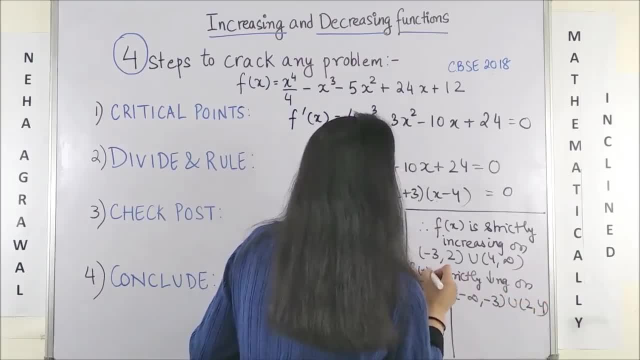 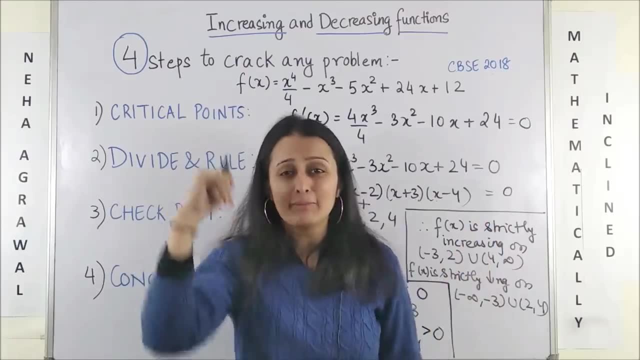 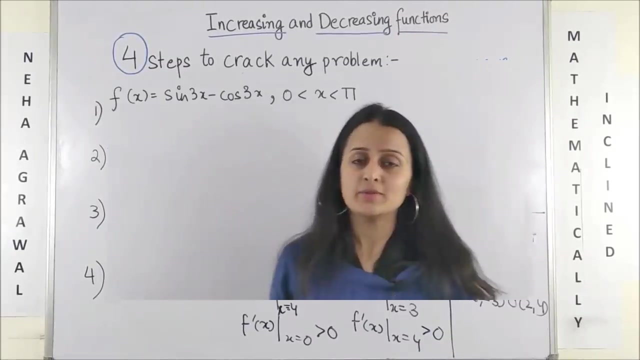 to 4.. So fx is strictly decreasing on these intervals. Kyun ban gaya na ye question. Bachcho ka khel. Make a note and then we move to another question. At times we get extra lucky and get extra lucky. sometimes we get extra lucky and get 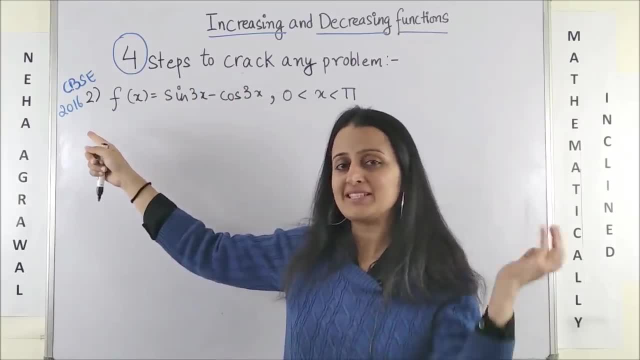 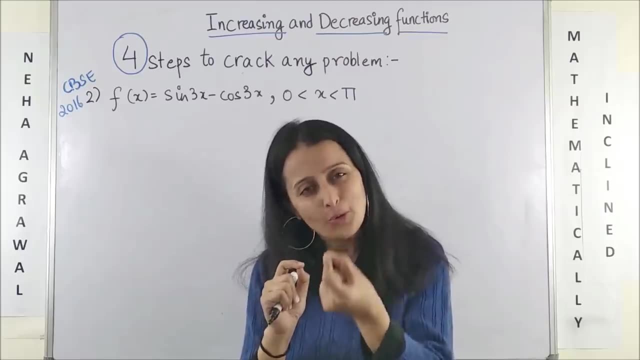 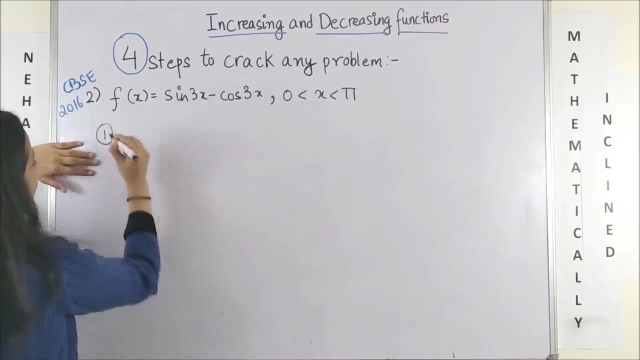 the same question for 6 mark, like it happened in CBSE 2016.. Still, we will follow the 4 steps. Then why is it 6 marks? Because trigger is a little tricky. How is it tricky? We will find that out. So, first of all, following our steps. step number 1 was critical points. 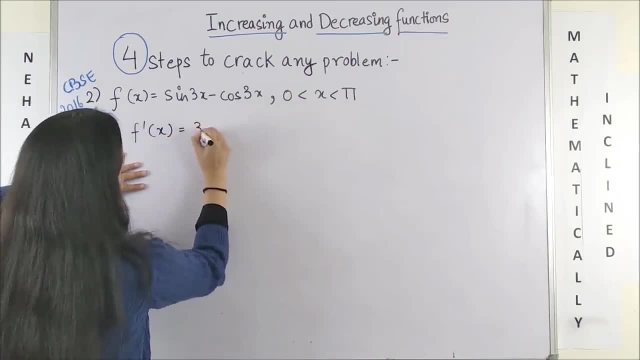 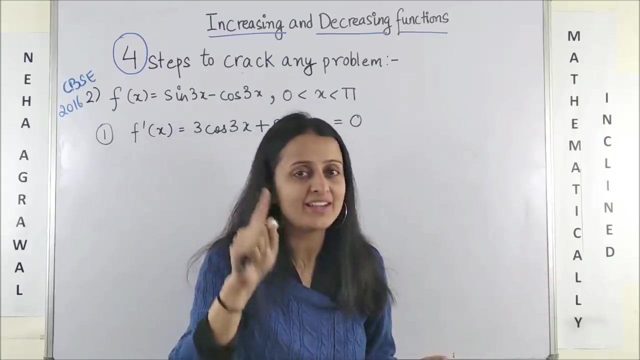 So f dash x is equal to 3 cos 3x minus. so that makes it plus sin 3x is equal to 0.. I am applying chain rule over here. In order to know chain rule, go to the playlist on differentiation. you will find the video. Okay, now putting this to 0, this means and: 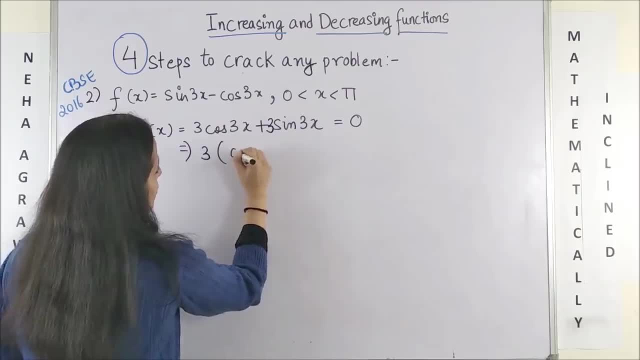 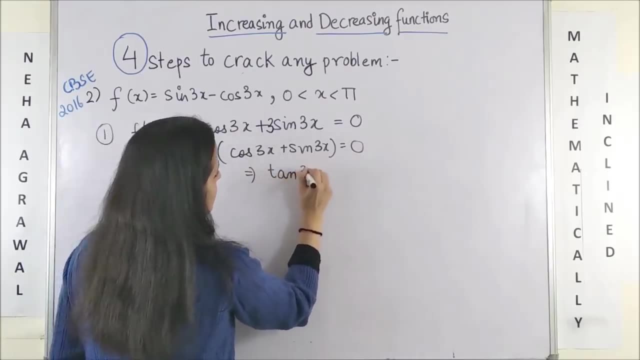 obviously I will have a 3 here. So thrice of cos 3x plus sin 3x is a 0. This means I can say tan 3x is minus 1.. Okay now, when is tan 3x negative? This means I. 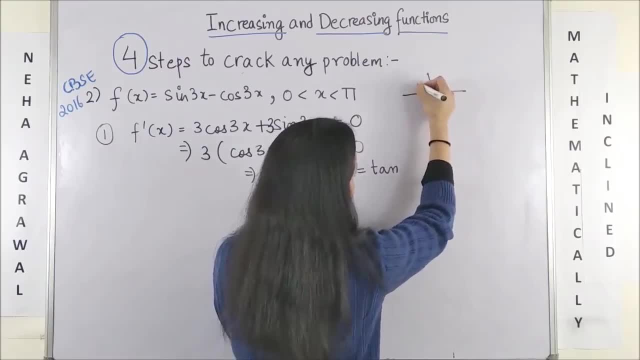 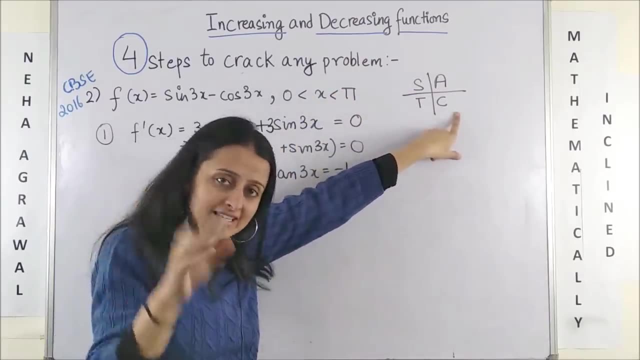 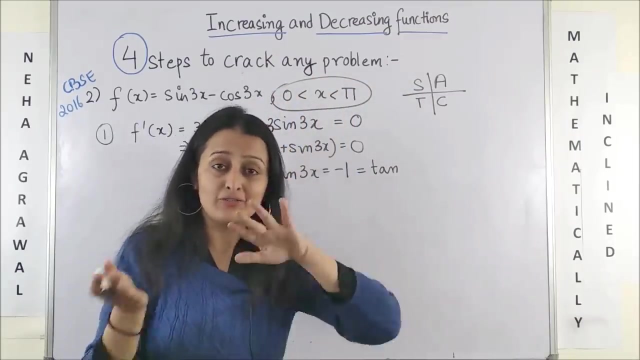 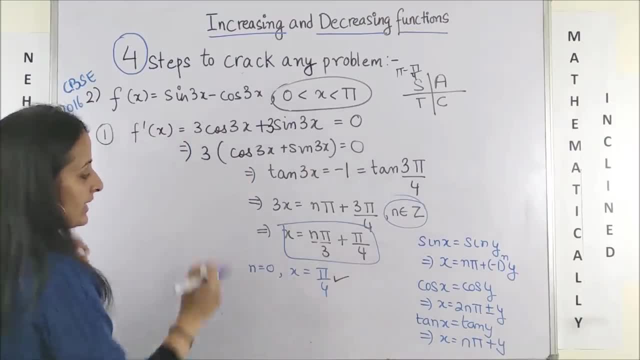 here I can take this to be 0 and 5.. So here I can take this to be 0 and 5.. So here I can. so yes, this is a critical point. Next, if I put n as 1, I get. x is equal to pi by 3 plus pi by 4. 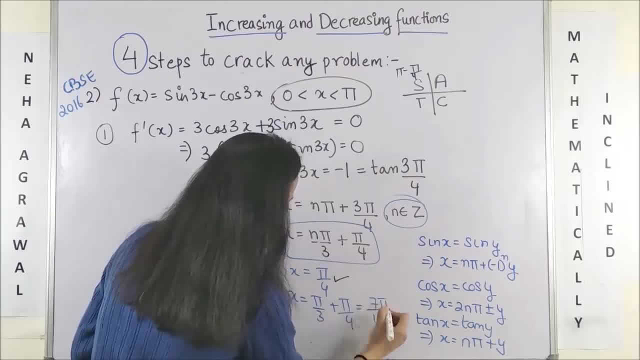 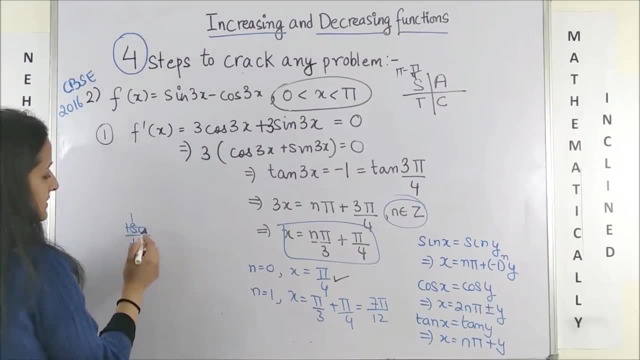 right, which becomes 7 pi by 12.. Now pi by 12 means 180 by 12.. If you actually see, this is 15.. So 7 into 15 makes it 105 degrees. Definitely lies between 0 and 180.. So okay, I accept this. 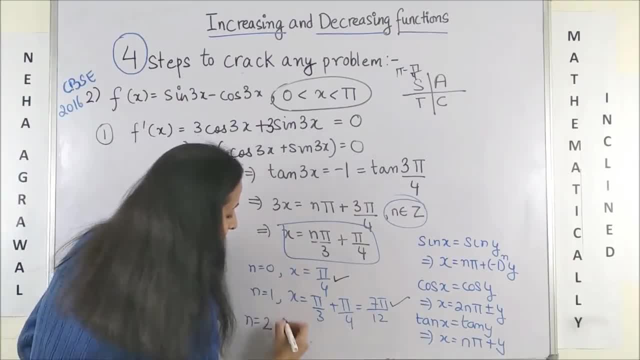 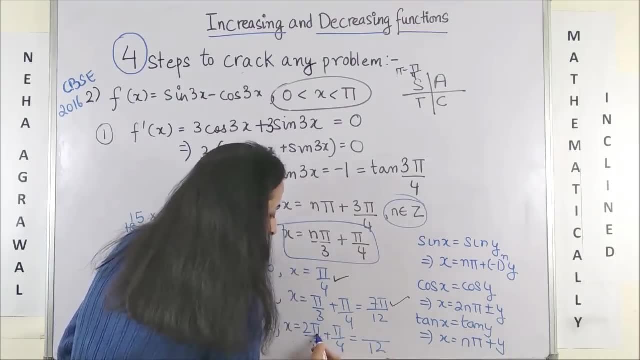 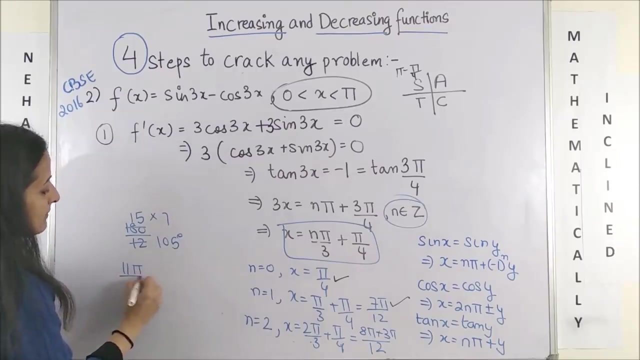 also. But when I take n equal to 2, this gives me x is 2 pi by 3 plus pi by 4, which means 12.. This is 8 pi plus this will be 3 pi, which means 11 pi by 12.. Now, if you put 11 pi by 12, 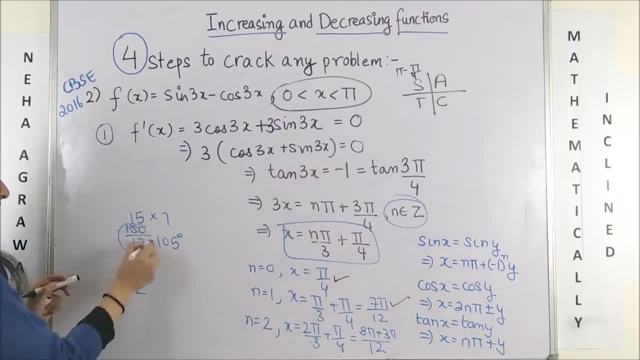 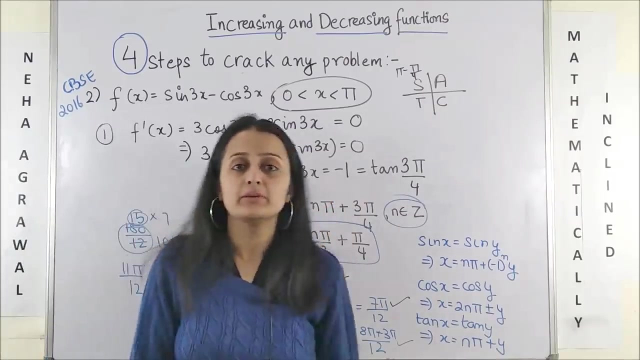 by 12.. Pi: 180 by 12,. this we have already calculated was 15.. 18 into 15 gives me 165 degree. Yes, absolutely, This is also in. So if you had said directly: 3x equal to 3 pi by 4,. 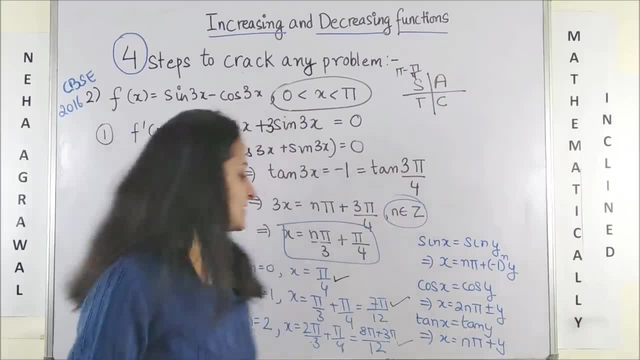 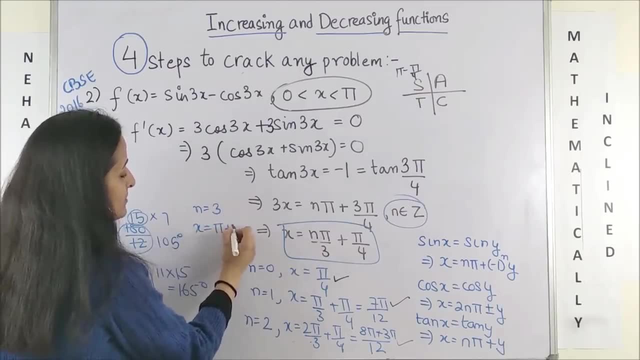 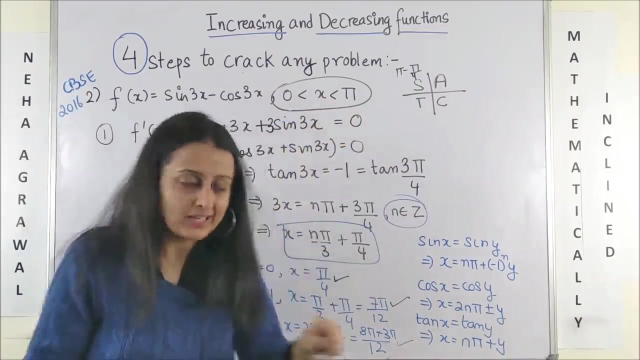 then you would have missed on so many critical points. Now, if I try taking n as 3, that makes it x as pi plus pi by 4.. Definitely not, because pi is a critical point. So after this I don't take any more, Okay. And same way, if I try taking n as minus 1, we get 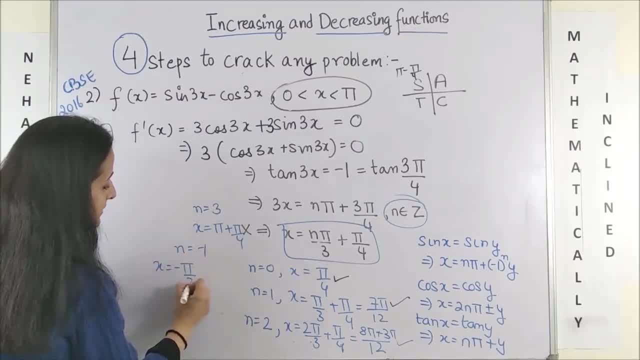 from here we get x equal to minus pi by 3 plus pi by 4.. So when I take the LCM we get minus 4 pi plus 3 pi, So minus pi by 12.. Again not applicable. So if I take n as 3 pi by 4, then I get minus 4 pi plus 3 pi. So 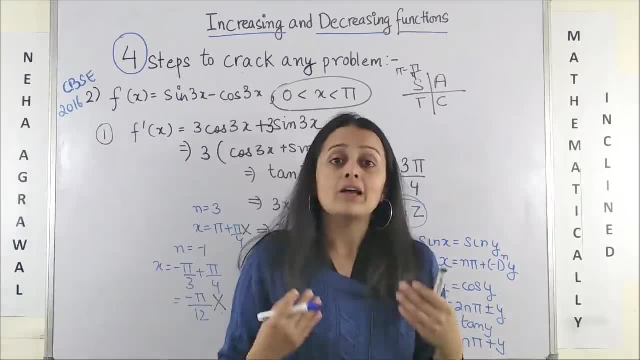 minus pi by 12.. So when I take the LCM we get minus 4 pi plus 3 pi, So minus pi by 12.. Again, not applicable. Reason being: I have my interval from 0 to pi. I know you feel this step is very. 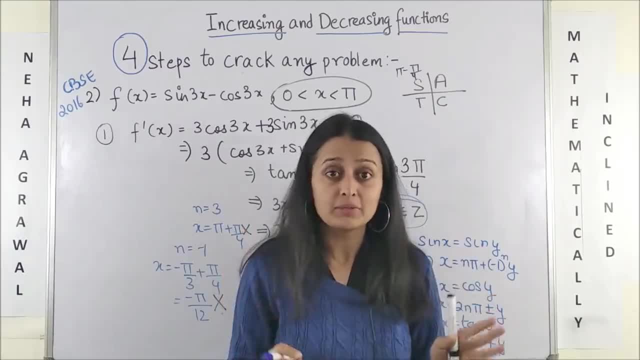 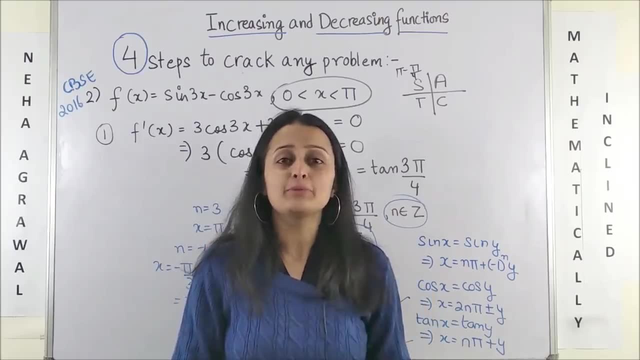 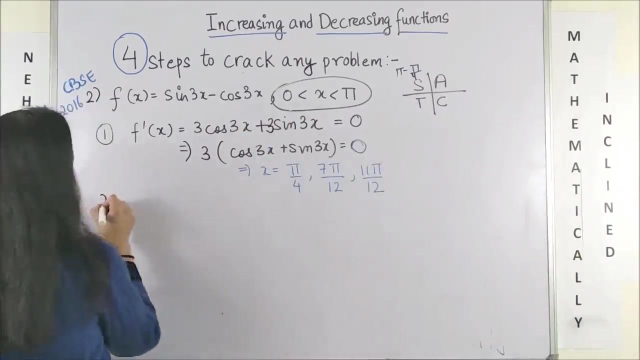 tedious, But if you remember these steps, toh bahut simple hai. And if it is a 6 marker, toh bahut 3 critical points toh bante hain. Make a note and then we proceed further. Okay, So now these are the critical points we got. So now, second step. 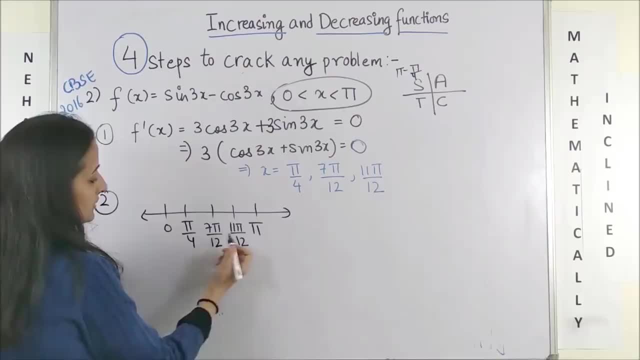 divide and rule. So I have split my entire interval into these. Now, if you feel you will get it right, then you will get it right. So you will get it right. So you will get it right. Confused, You can take them to be 45 degrees, 105 degrees and 165 degrees, So you know how to. 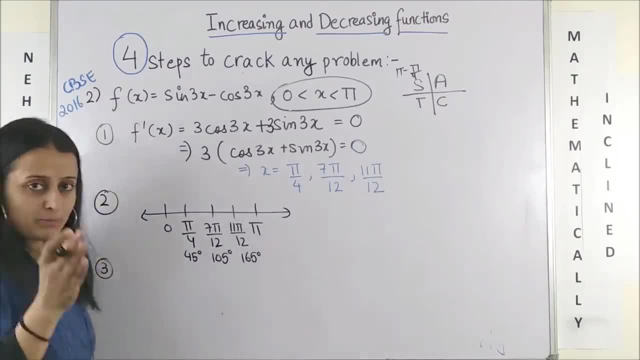 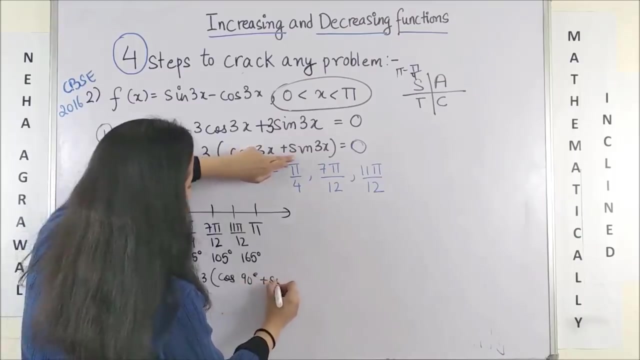 take the values Right, Step number 3, check post. So I checked for the signs F, dash x from 0 to 45.. Let's take x as 30 degrees 30 mein. kya hua? This becomes 3 cos 3 into 30. is cos 90 plus sign. 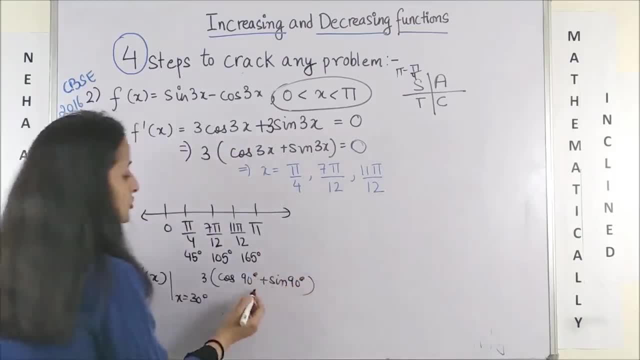 of 3 into 30 is 90 degrees. So in short, this becomes 3 cos 90 plus sin of 3 into 30 is 90 degrees. So in short, this becomes 3 cos 90 plus sin of 3 into 30 is 90 degrees. So, in short, this becomes: 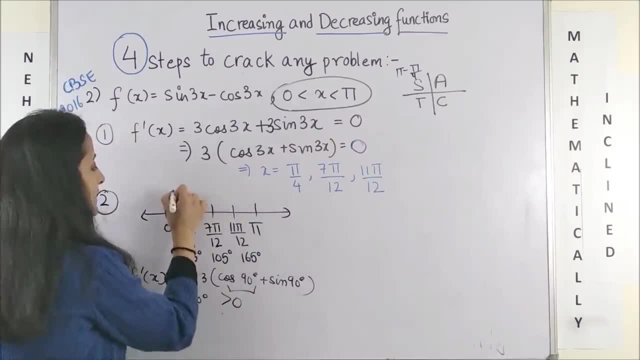 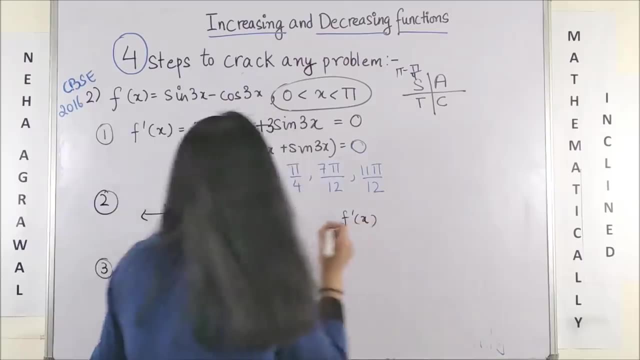 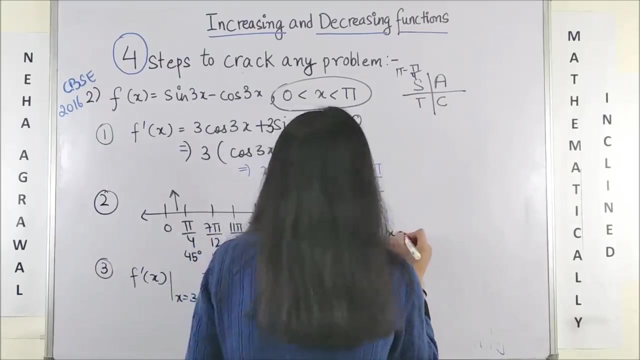 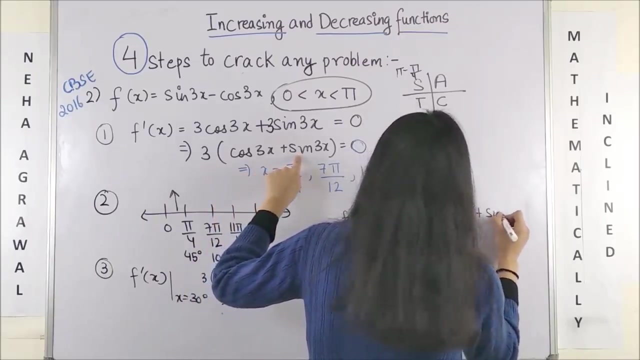 0.. I end up getting 3, which is positive, and thus this interval is increasing. Same way, moving to the next subinterval, I take f dash x. Now I want something between 45 and 105.. I know 60. Let's put 60.. So if I put x as 60 degrees, this becomes 3 cos 180 degrees plus sin. 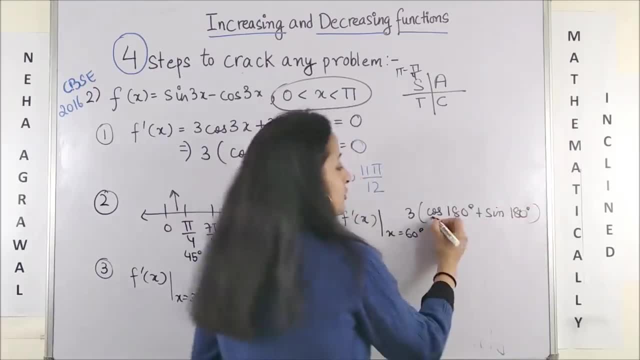 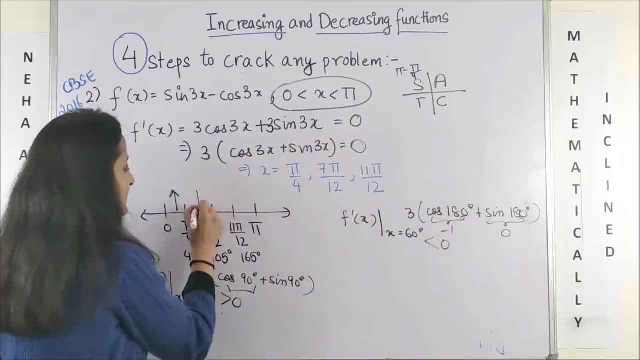 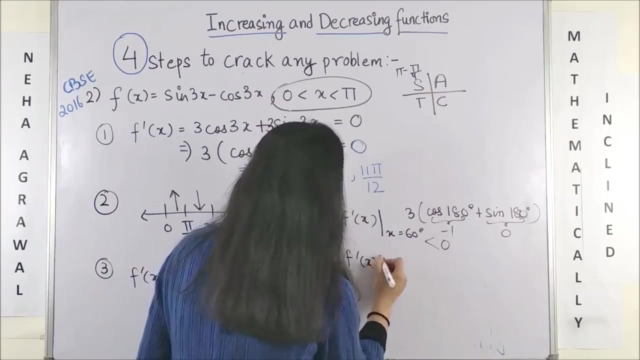 3 into 60 is 180 degrees. I know cos 180.. This is minus 1 and sin 180 is 0. So aagaya na Less than 0.. Okay ji, this is decreasing. Moving further, I want some angle between 105 and 165.. I know thoda tricky hai, but let's try to. 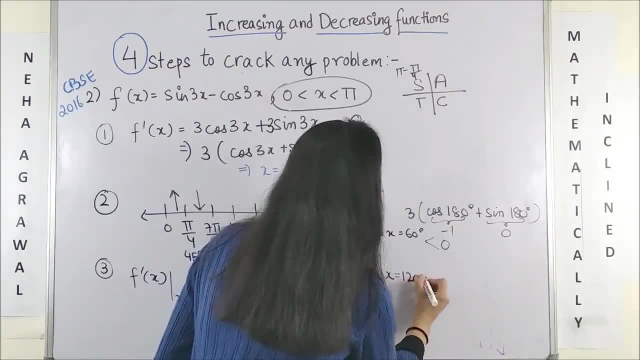 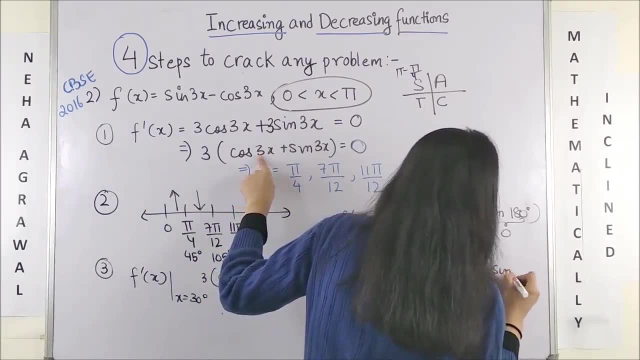 take something which is nearly the best. So let's say 120 degrees. Now this makes it 120 into 3.. So 360 degrees plus sin 360 degrees. Now we are going to take x as 30 degrees, So this becomes 3 cos 180 degrees plus sin 360 degrees. 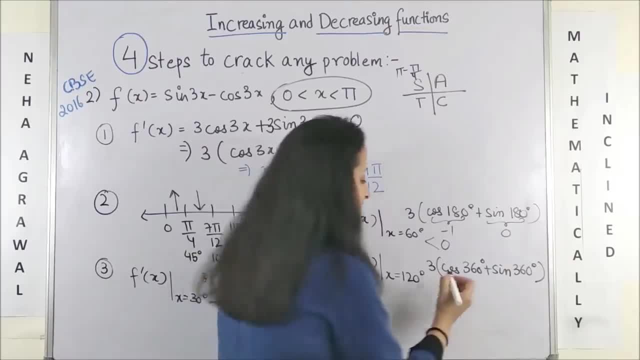 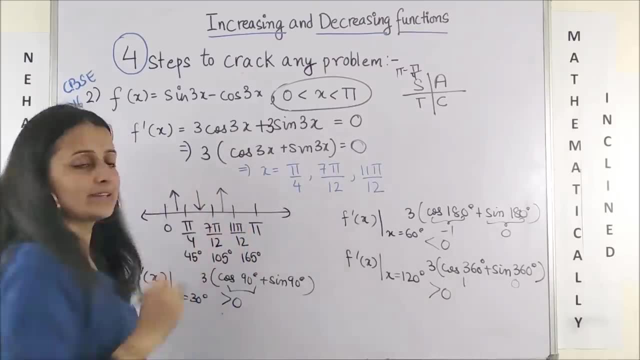 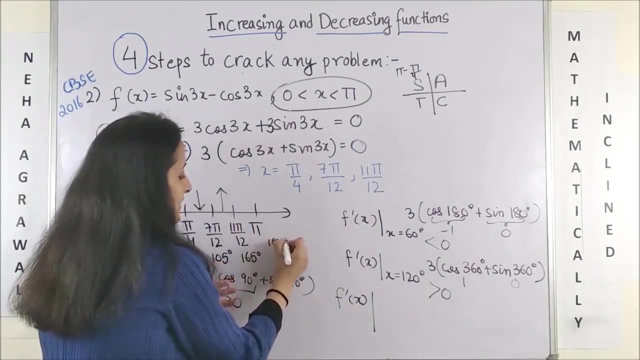 Now you all know, or you can of course find: cos 360 degrees will be 1 and sin 360 degrees will be 0.. So aagaya ye positive. The function is strictly increasing. Moving to the last subinterval, f dash x, Now 165, and this is 180 degree. But let's take anything random. 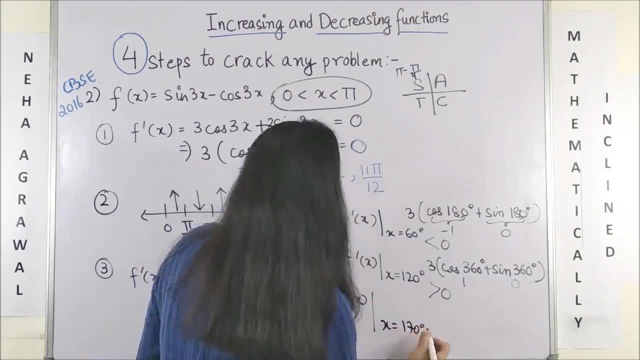 Let's say we take it as maybe 170 degrees. Okay ji. So here I put 3 cos, This will be 17 into 3.. So 4 cos 180 degrees plus sin 360 degrees, plus sin 360 degrees plus sin 360 degrees. So. 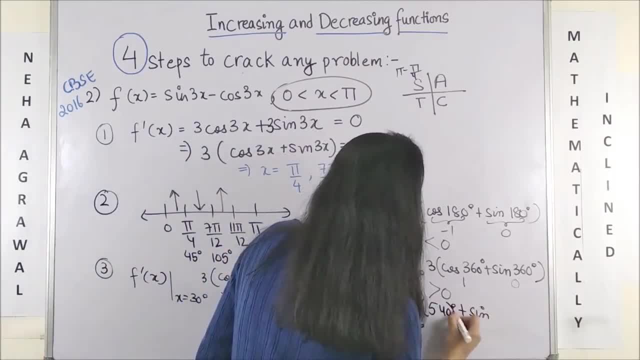 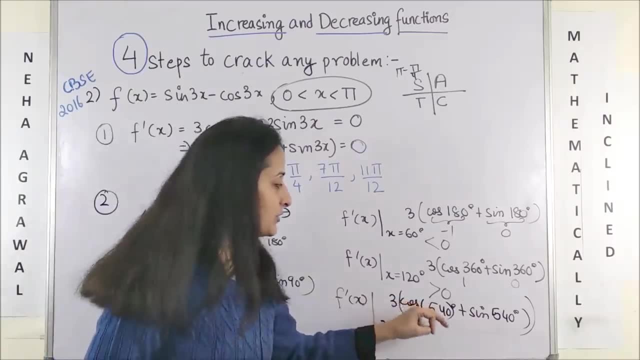 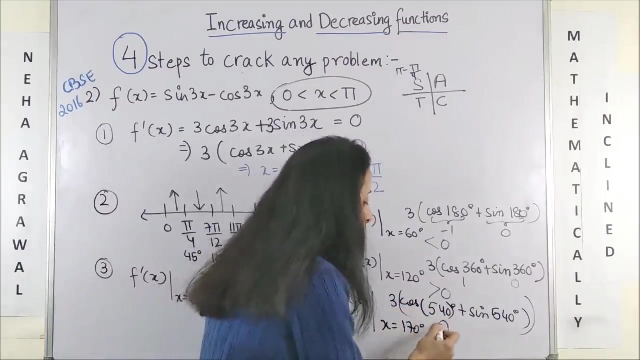 540 degrees plus sin 540 degrees. Right, This is what I have Now. you know it is an odd multiple of pi by 2.. So cos of this has to be 0 and sin of 540 degrees. You can calculate, it will turn out. 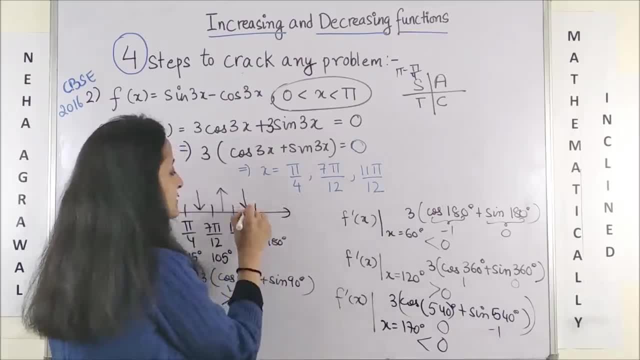 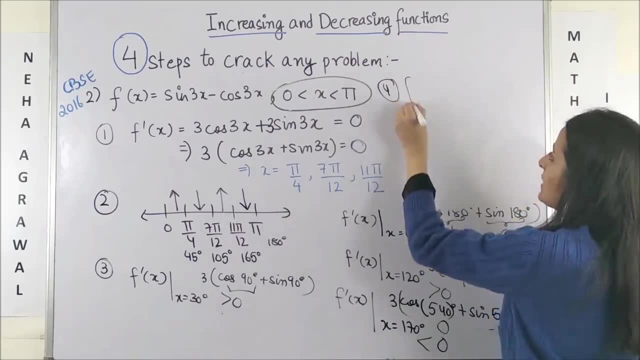 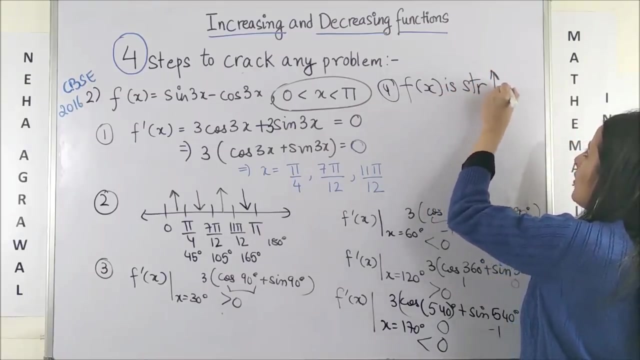 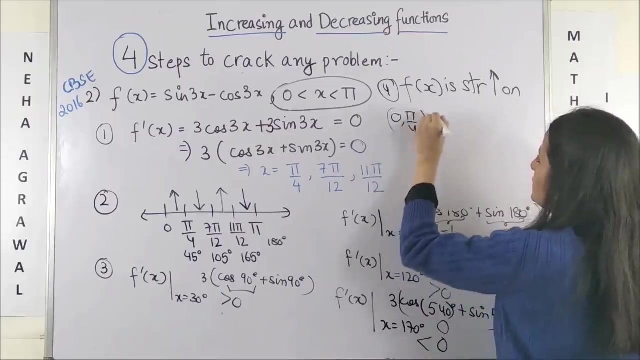 to be minus 1 and thus this is negative, So this is strictly decreasing. Now, finally, I have the last step, which is the conclusion. So I will simply say that my fx is strictly increasing on the subinterval which is 0 to pi by 4 union. I have 7 pi by 12 to 11 pi by 12, and strictly. 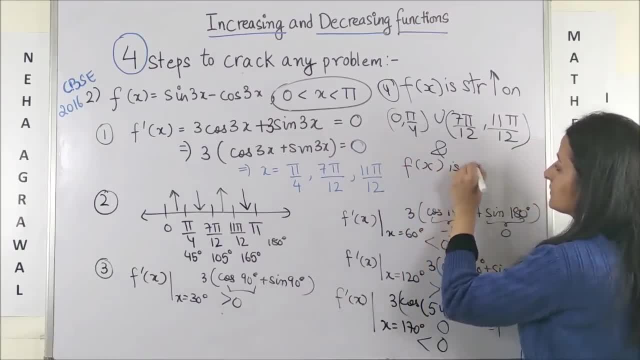 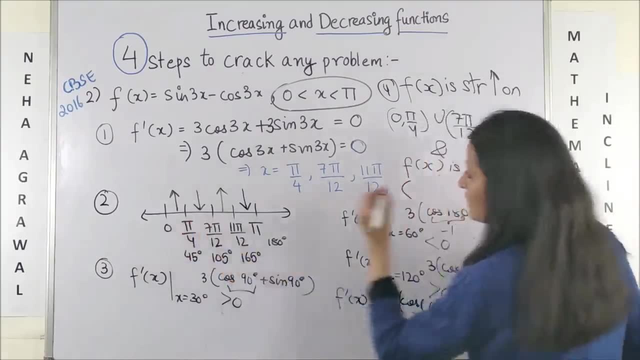 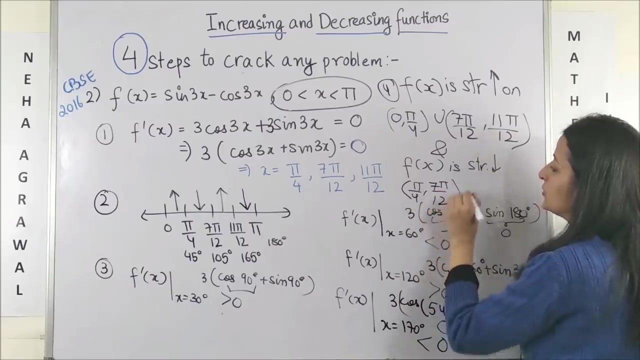 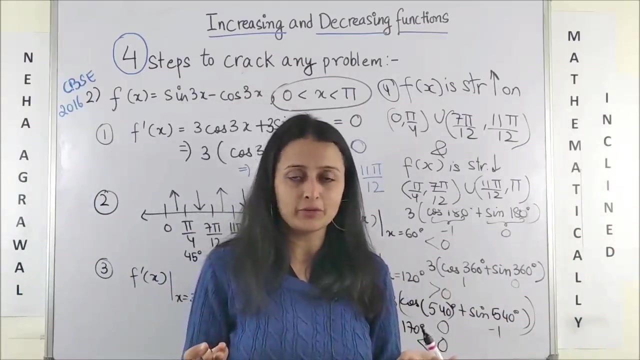 decreasing on. we will have pi by 4 to 7, pi by 12, union 11, pi by 12, 2 pi. Trust me, Right now it appears to be a lot of calculations, but if you do it on your own it doesn't take so much time. So please make a note. 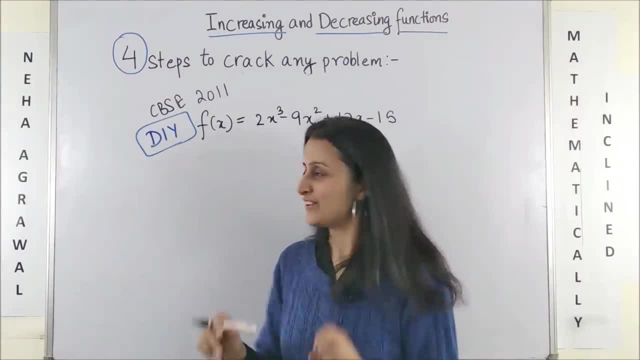 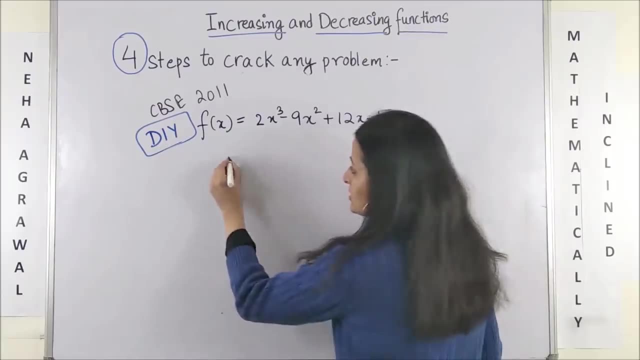 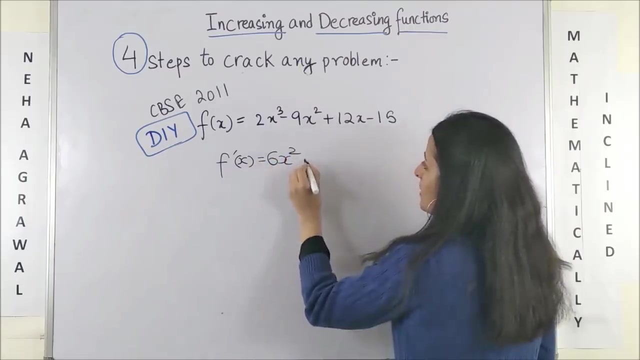 Now it is time for our chotu sa do-it-yourself question. This came in CBSE 2011.. Now your simple polynomial function- you know your f dash x is equal to this- will be 6x square minus 18x plus 12.. Now for critical points. 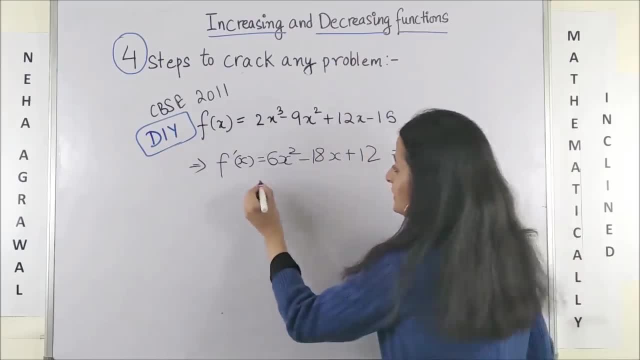 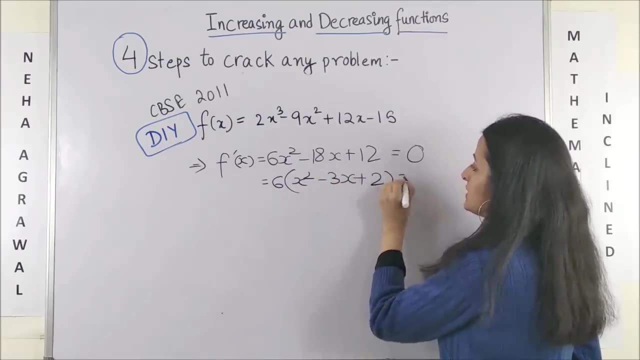 equate this equal to 0.. Okay, If I take your 6 common, we are left with x square minus 3x plus 2 is equal to 0.. Okay, So here this is what I get Now in order to factorize this. 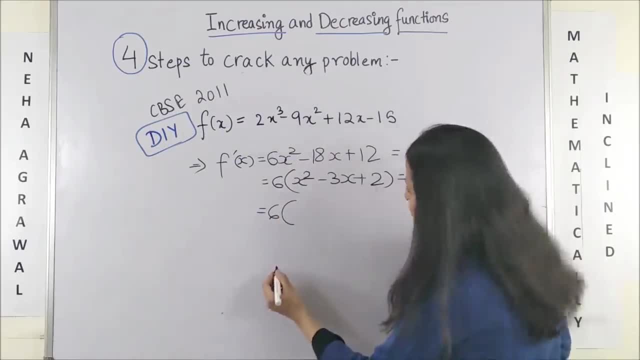